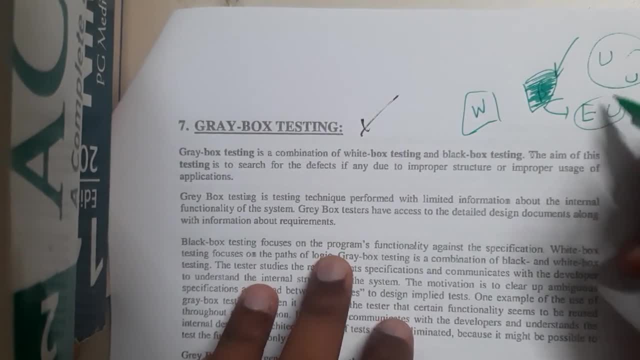 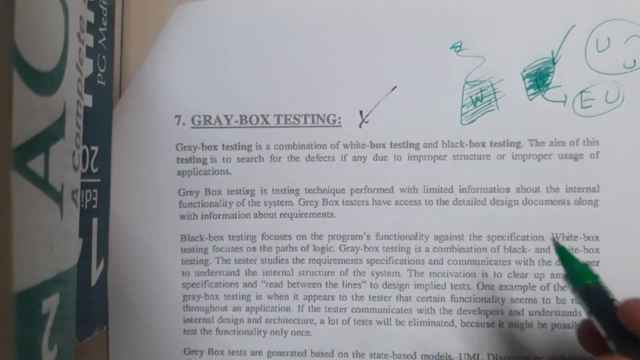 be just giving his required input and he will be getting his required output. So that concept is nothing but black box, Whereas white box that he. this is mostly done by the developers, So the developer knows the exact logic, right. So if he is giving value x equal to 10.. So he knows where. 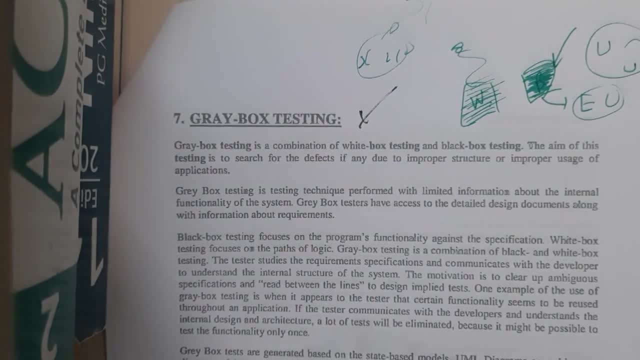 this x will travel in, how many calculations will be done, How it will travel. Everything he knows. So he knows the exact logic, right. So if he is giving value x equal to 10. So he knows where and he can see everything transparently right. So that is the reason why it is called as white box. 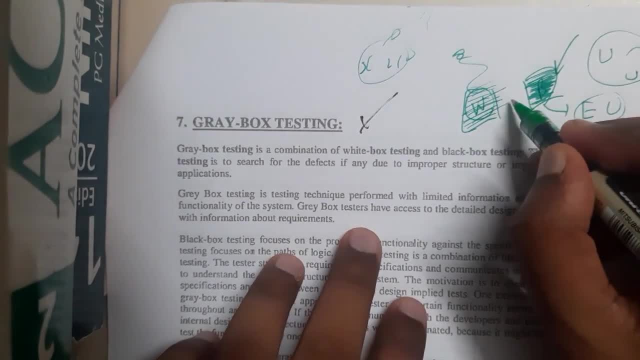 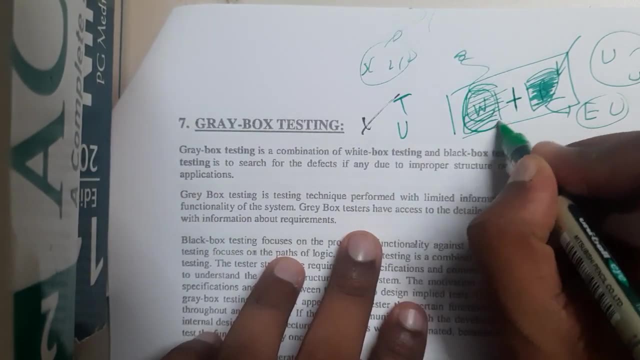 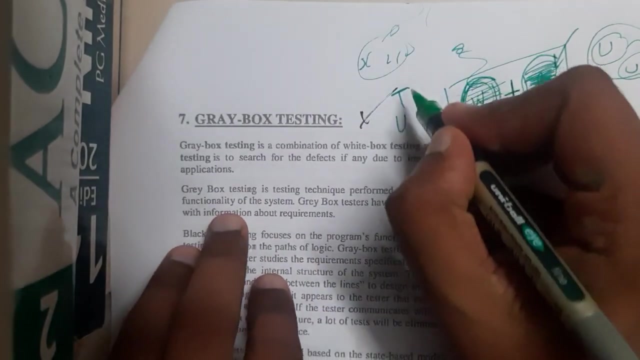 testing. So now gray box testing. So what is the gray box testing? It is nothing but the combination of both guys. So here the user or the tester will have the idea about what is the internal logic exactly and what is the expected input and what is the expected output. So here both the advantages. 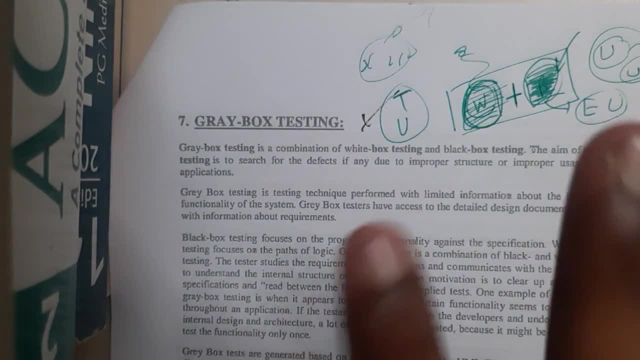 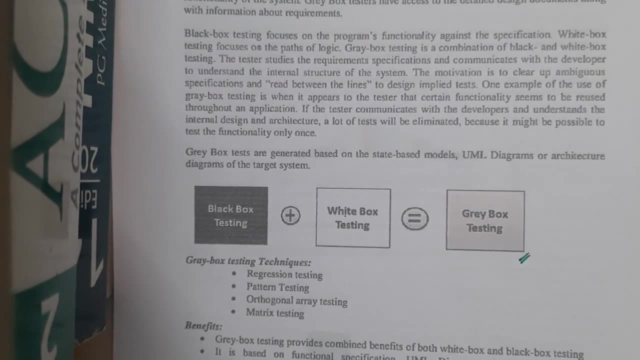 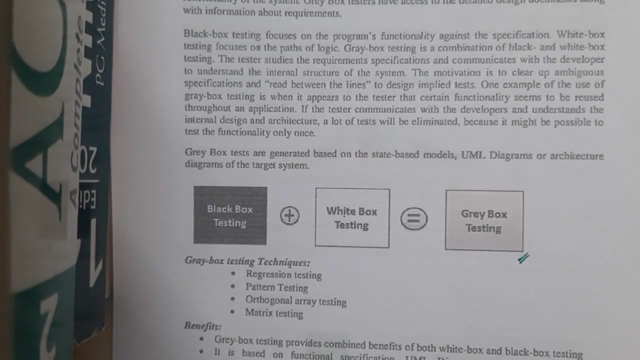 of both those methods are combinedly taken and built a method that is called as gray box testing. So you might be saying that, okay, so that sounds really good, but are there any major advantages? Okay, so assume that you created a software. Okay, so you want to test it in a proper and efficient 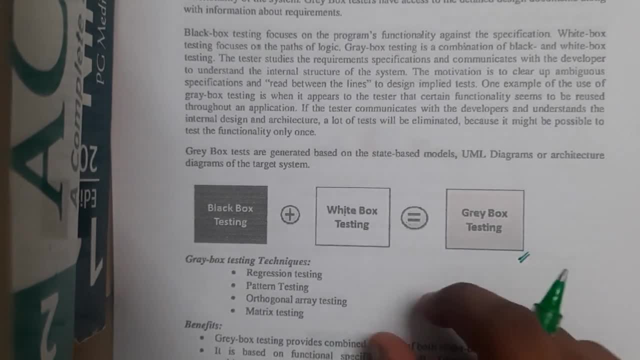 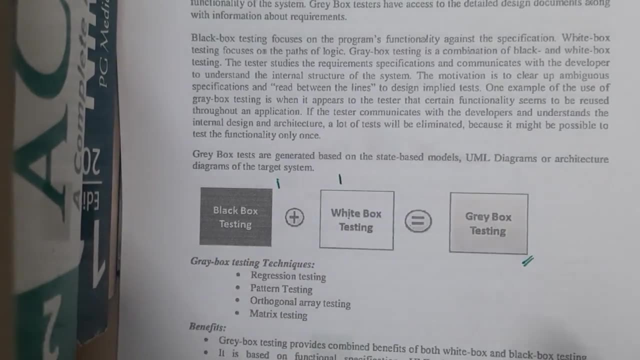 way. Okay, so in this situation, whom you will be giving? you will be giving one copy to the black box and one copy to the white box testers, right? Yes, so assume that this is done by one person and this is one done by one person. So, basically, to perform those two operations, you need two persons. 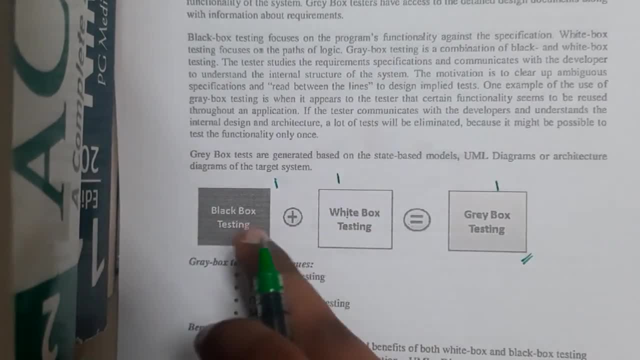 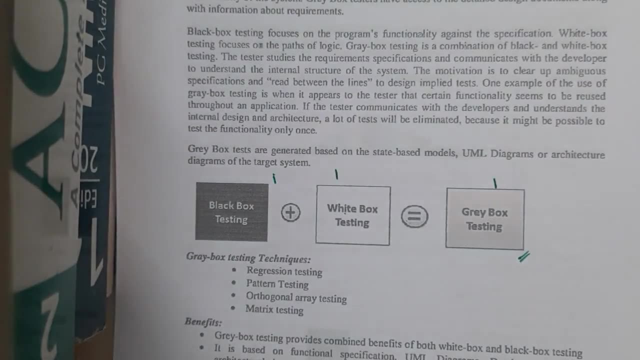 Whereas if you are using gray box testing, only one person will do Those two issues right. He will test it with respect to inputs and he will test with logic. So if there are any issues, he will report you. and the major advantage of gray box testing is: 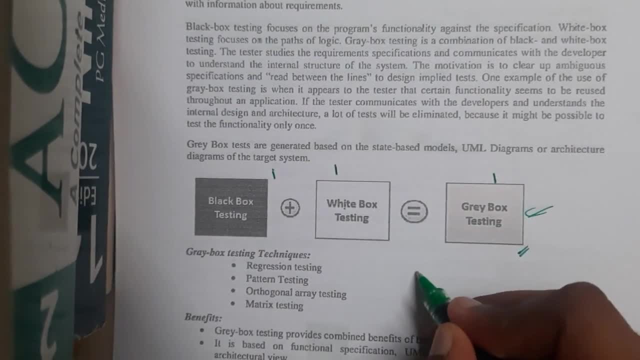 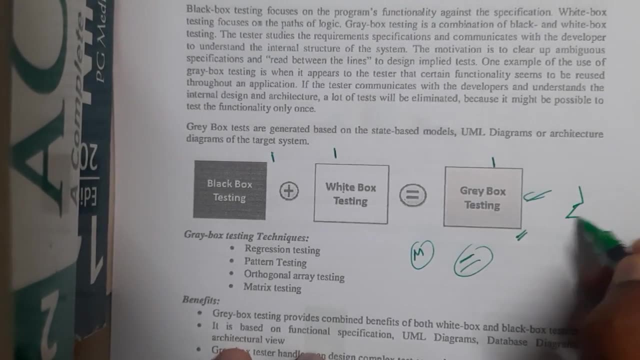 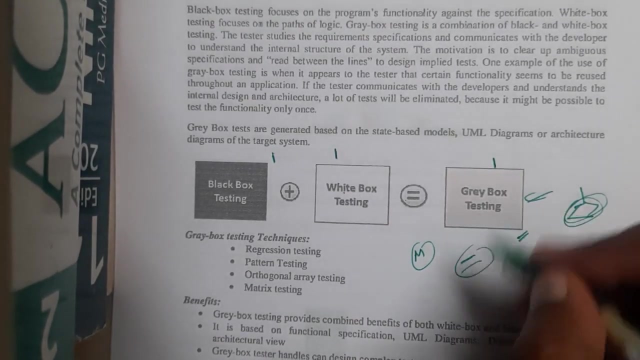 as he knows the back end logic. Okay, so he will say: in that particular module, in that line you might have written the error or in this particular flow the decision is not working properly. So he can identify the things because he is a developer, right, Indirectly, he is a developer, So that is. 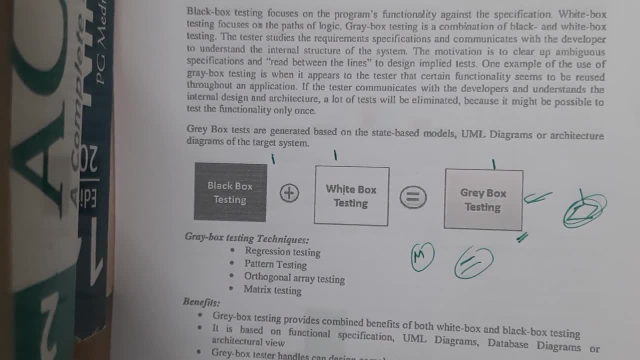 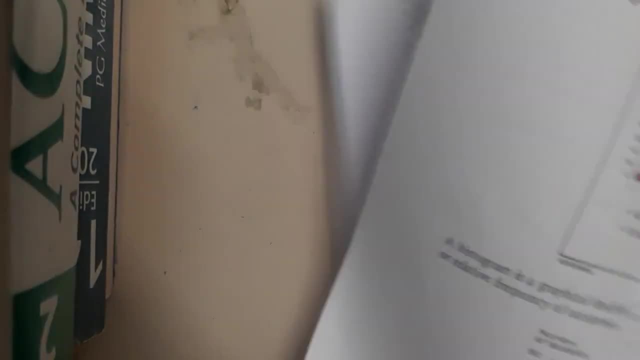 the major advantage of gray box testing guys. Okay, yes, so I hope everyone got some basic idea about the gray box testing, right? Yes, so please go through the theory, guys. It will take around five minutes for you to read, So please make sure you.